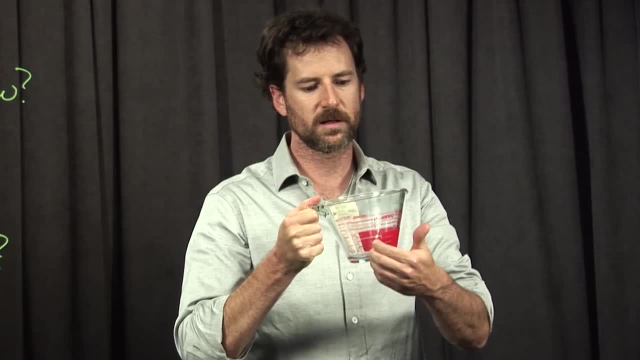 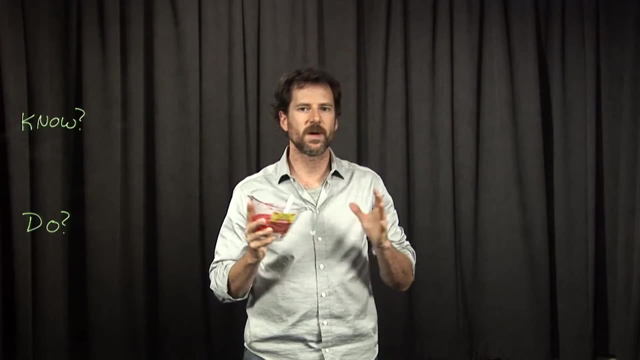 that if you hold them right-handed, you see English units and if you hold them left-handed, you see metric units. So, to summarize this, measuring cup redesign gives us a couple of important lessons. For starters, if we simply ask people what they want, 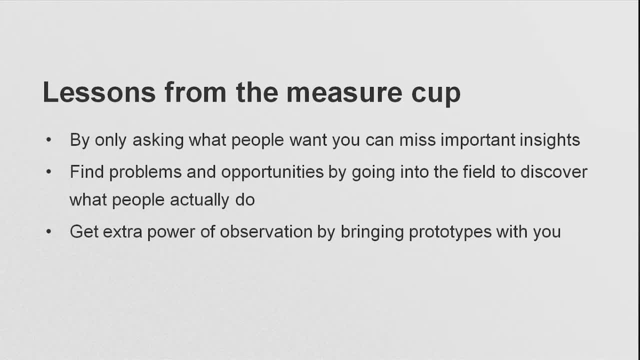 we might miss important opportunities. Second, there's real value in going out into the field and gathering behavioral measures, as opposed to just asking people. The third is that when you go out into the field, bring along a prototype, because that'll change the interaction. 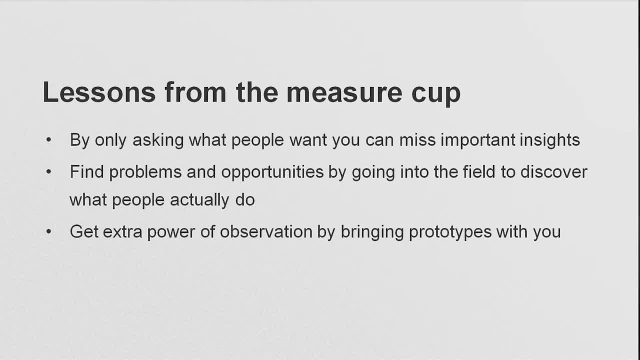 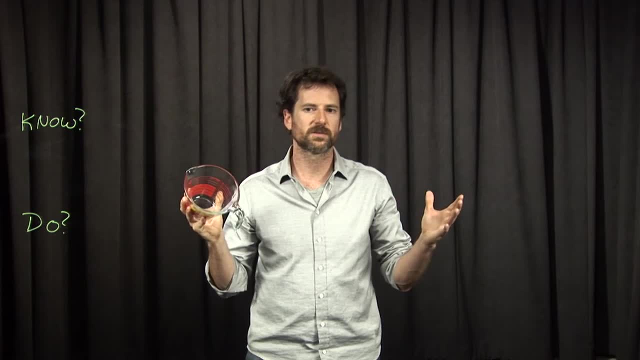 And the fourth is that the world is full of people who are tinkering in their garage and that, when the stars align, we can bring together these diverse talents to offer a new, exciting user experience for the world, With measuring cups like all user interfaces. 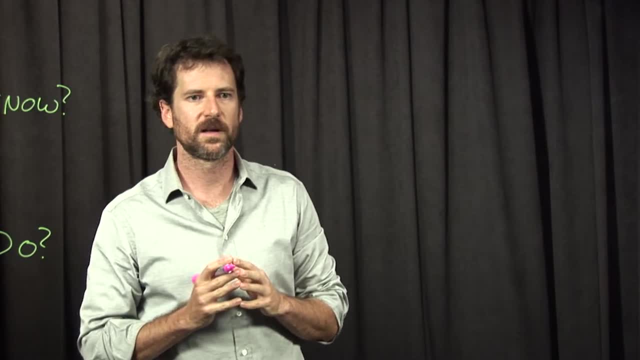 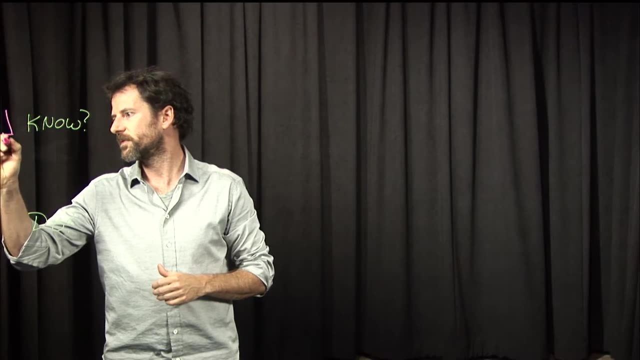 there are two fundamental questions that we want to ask, And I'd like to share with you a drawing that I got from my colleague, Bill Verplank. Bill points out that really we've got these two main questions. The first is that when I encounter a measuring cup, 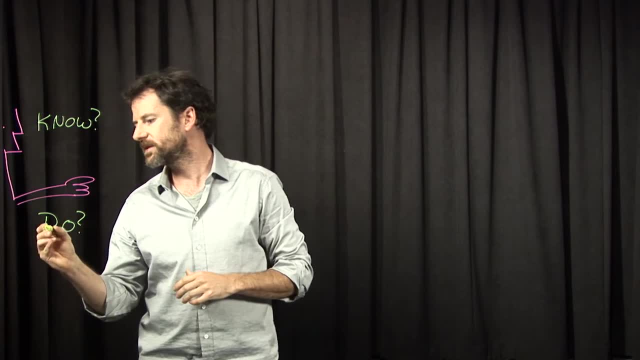 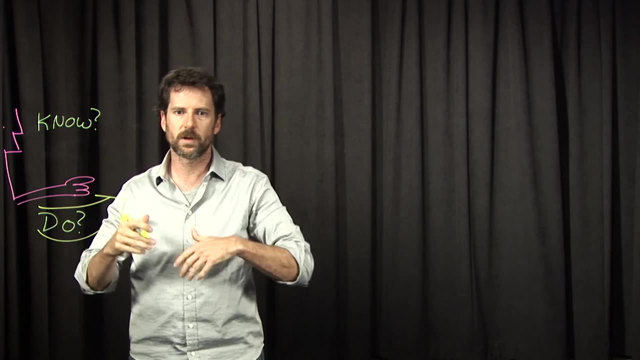 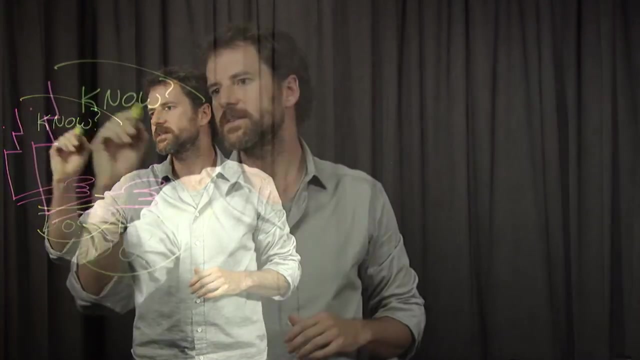 or a new computer software or anything else. I need to figure out what is it that I can do. Then, after I do that, fill the liquid, try to print a document, retrieve something from the internet- then I need to figure out what is it that happened. 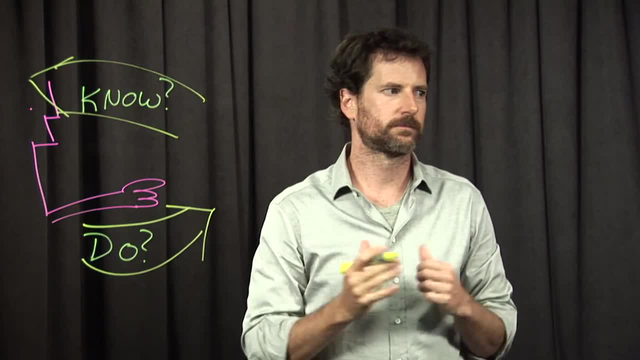 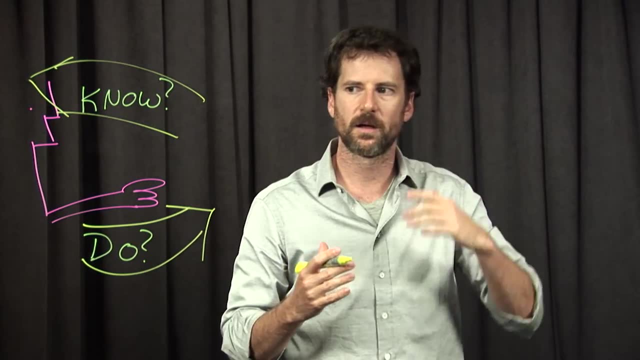 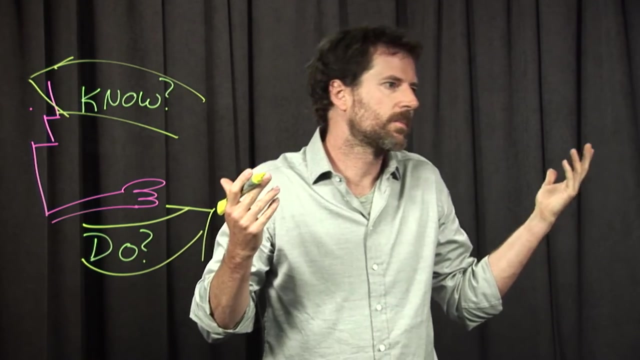 And so the interface is teaching me. how do I know? One of the great insights of cognitive science is that if you understand what's in people's head, you can do a way better job of explaining their behavior. We're going beyond, oh well, the user's dumb. 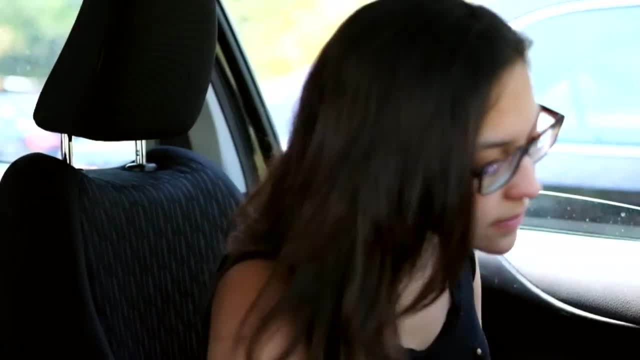 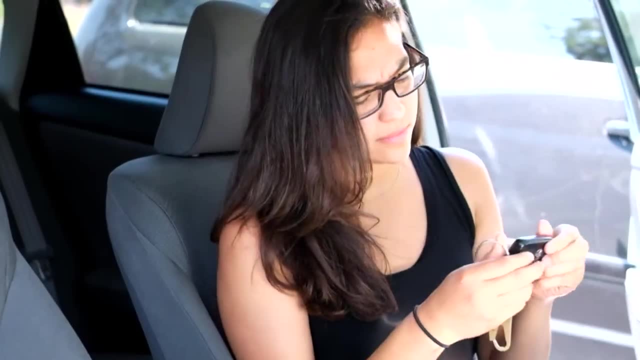 to well, if they did that, then they must be thinking this: I'm used to driving a normal car that you start with a key that you put in the steering column. Recently I got a rental car, got into the driver's seat, had keys. 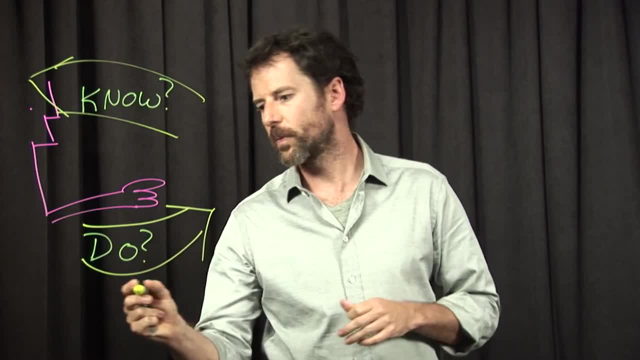 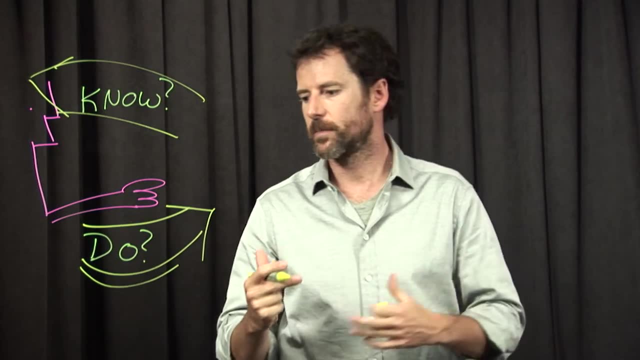 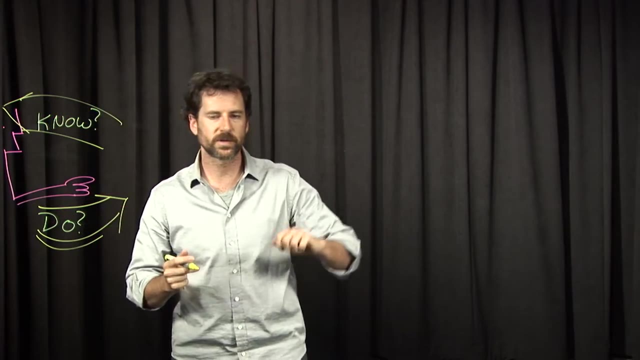 but there was nowhere to put them. That's an example where I didn't know what I how to do. You can see that my experience taught me what I should expect, but my expectation was violated by the newfangled car experience. Similarly, once you do get the car started, 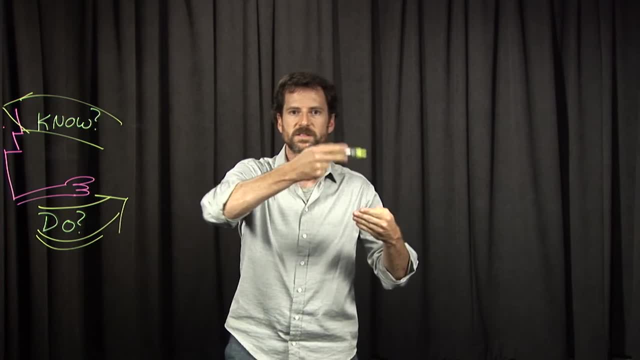 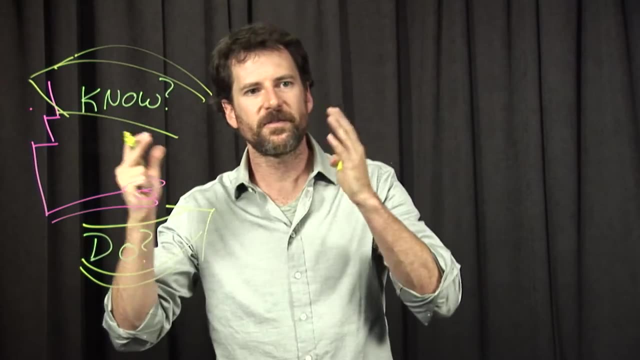 how is it that you know that you achieved it? Well, you might see the RPMs on the tachometer go. you might hear the engine lights might come on. You're getting that feedback which informs your mental representation of what just happened. 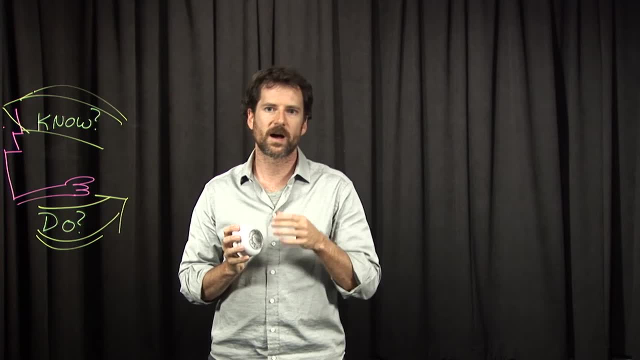 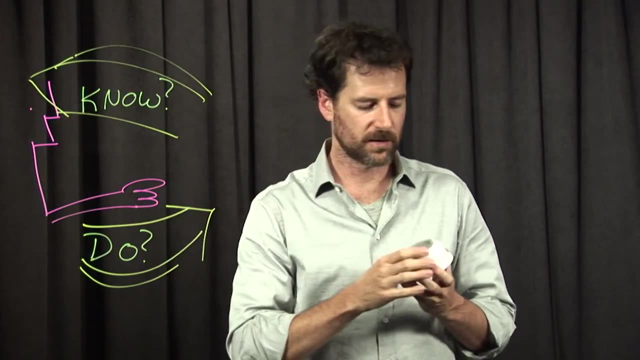 Here's a wonderful example. This is the classic Honeywell thermostat designed by Henry Dreyfus. What I like about this, from the perspective of our actor right here, is that when I ask the how do I do? question, I'd like to set the thermostat's temperature. 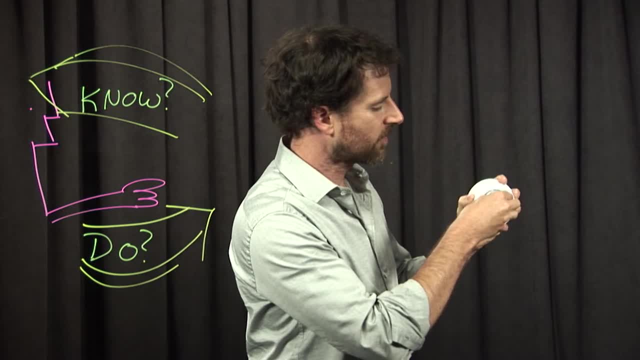 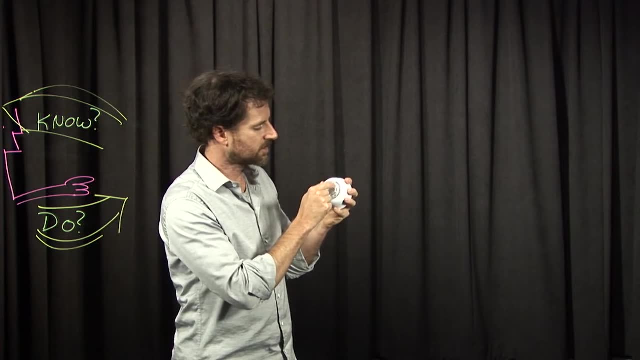 it's pretty easy. It's really obvious. Right on the front there's a strong signal that there's a dial I can turn. I know that because it has these ridges. it's got an indicator here and when I turn it. 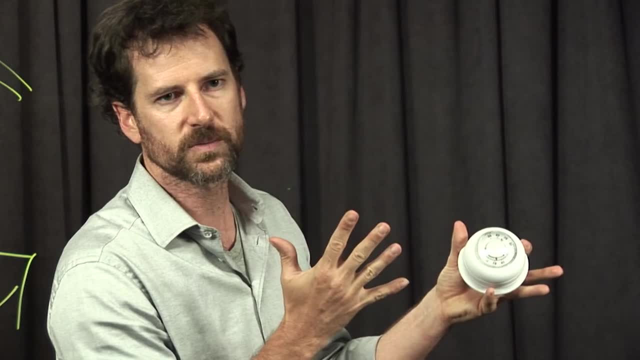 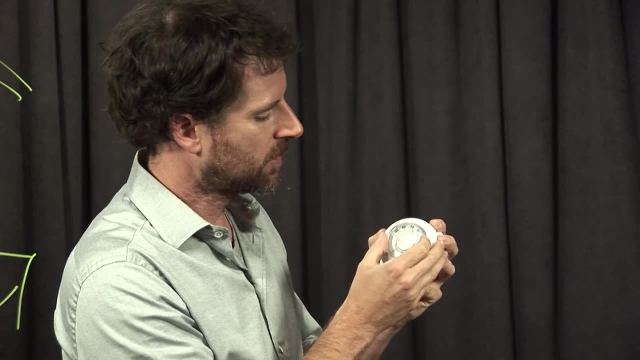 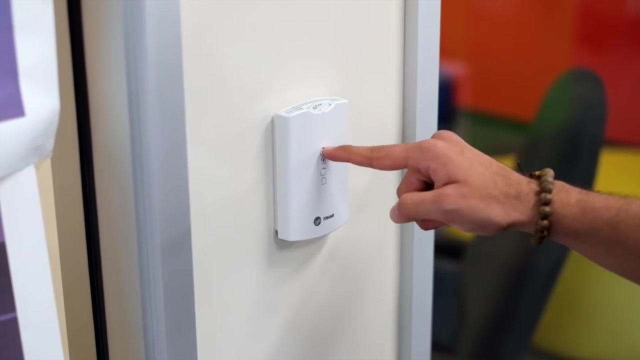 I get direct, immediate feedback, what in computer terms we now call direct manipulation- And that feedback is tied directly on top of the output. You want it 60 degrees, 70 degrees, heck 80 degrees, no problem. For many years, thermostats moved away from this more direct manipulation approach. 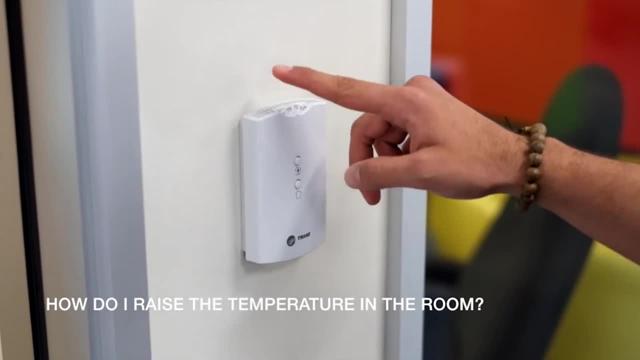 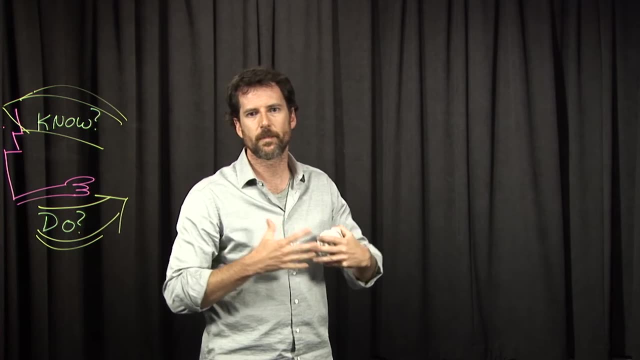 to have buttons or other things, and that indirection, like with VCRs and other electronics, made things actually a lot harder to use. And more recently we're seeing this directness come back into information appliances, The Nest thermostat, for example. 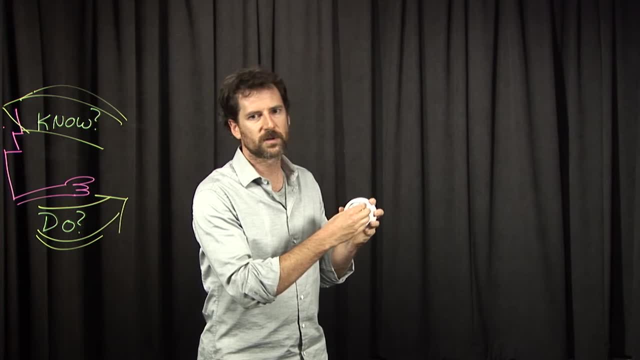 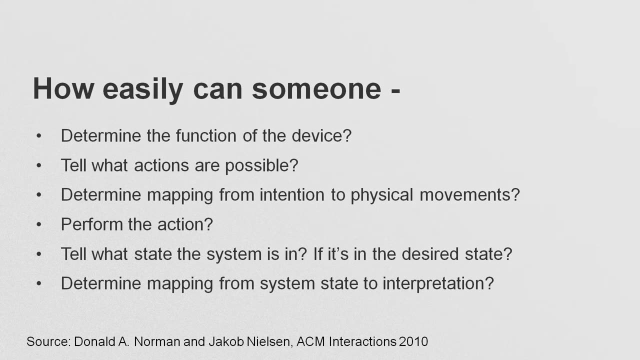 in many ways is paying homage to this wonderful classic Dreyfus design. Don Norman and Jacob Nielsen give us some really useful questions as designers for being able to figure out whether the interface that we're creating will be natural and easy to use, And I'll leave these here for your own work. 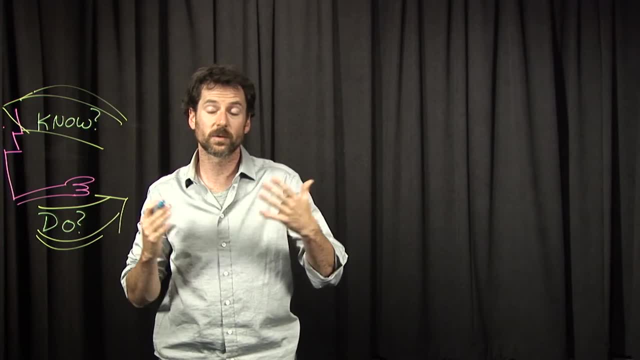 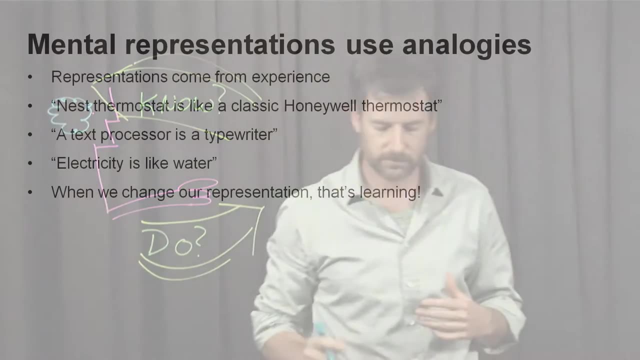 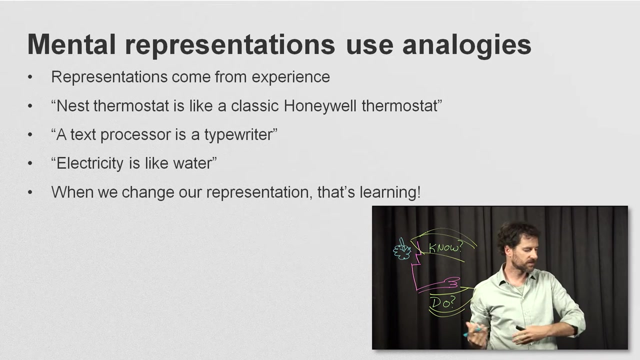 People obviously behave differently depending on how they think the world works In our minds. we build these mental representations. Often the representations in our minds are using analogies that come from experience. The Nest thermostat is like the classic Honeywell thermostat When I'm writing a computer document. 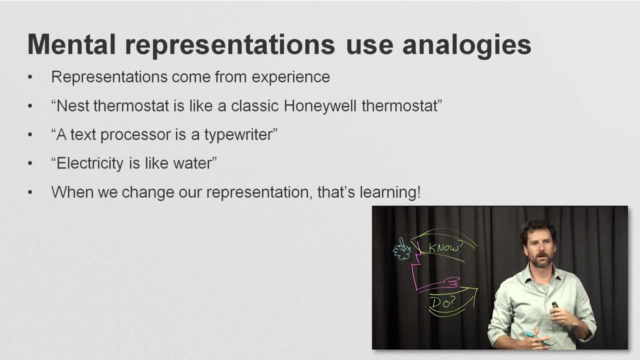 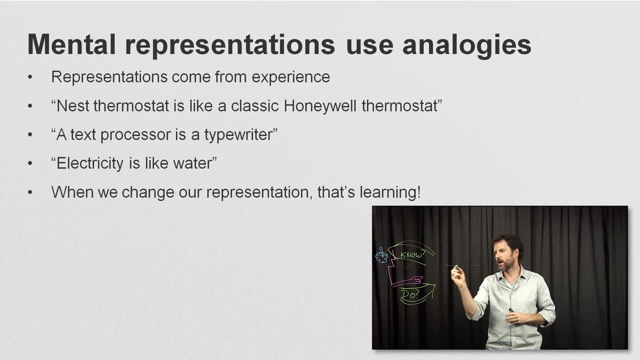 that's like using a typewriter. If I want to explain how electricity works, I might explain it by analogy to water: that the wires are pipes, where bigger pipes allow more water or electricity to be carried, that there are reservoirs or capacitors. 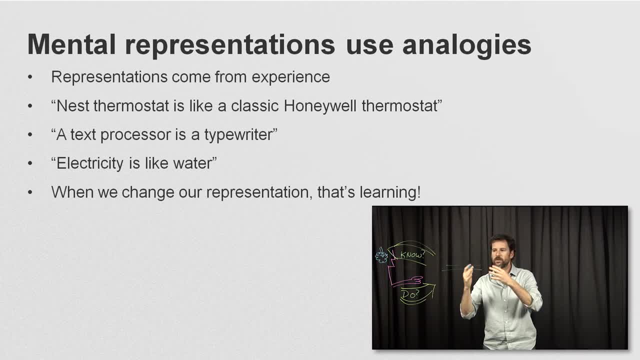 and a lot of basic principles of electricity. you can explain using the water analogy. That's not to say that everything is neat and tidy upstairs. Our mental models often aren't right. They're almost never right. They're never complete. Electricity is like water in some ways. 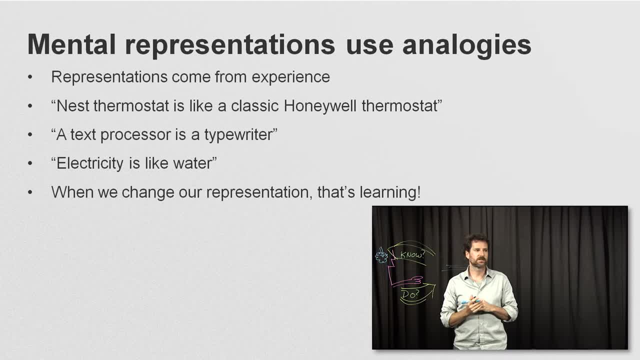 and not like water in others, And they're often rife with superstitions. Computers are an amazing catalyst for superstitious behavior. We all have these superstitions. even really technologically savvy people that we know in some level aren't real. 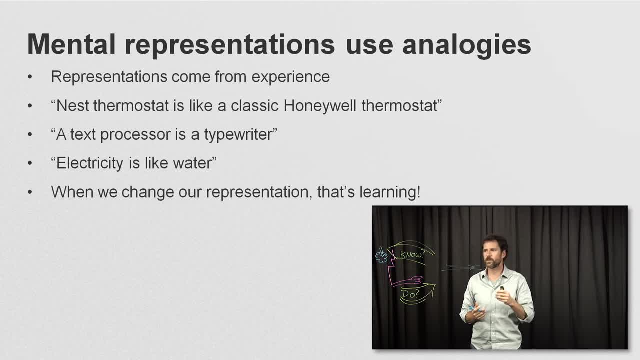 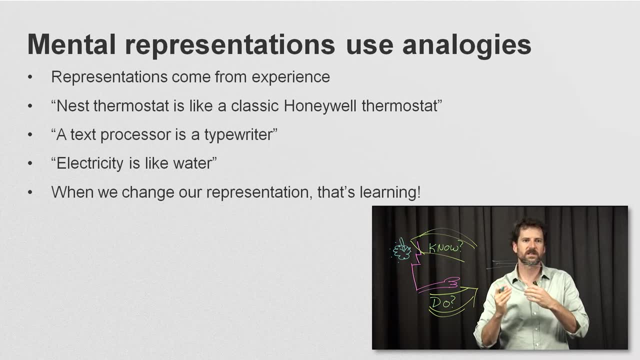 and yet, because we don't have a better explanation, we use them anyway. Over time we build more and more representations. These can dovetail together, so I can think that electricity is like water and might be like teaming crowds in another way. 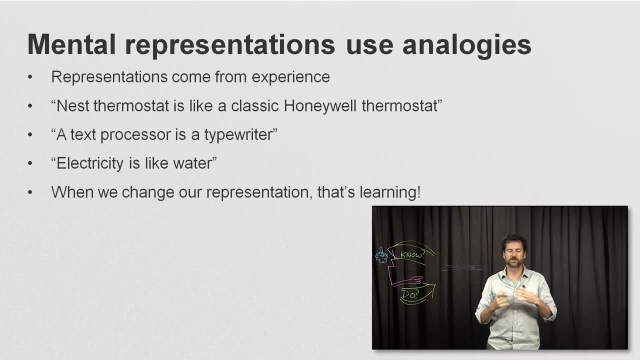 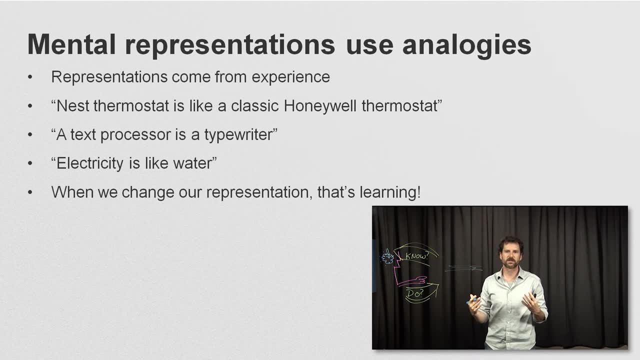 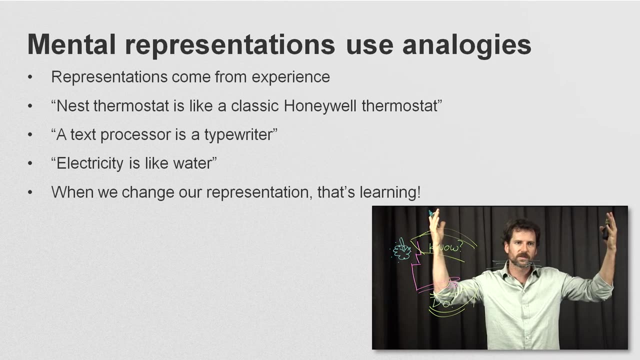 or I can layer on more abstract representations using equations. They coexist at the same time When we change or add our representations. in many ways, that's actually what learning is. It's this accumulation and evolution of our mental representation set The goal for you as the designer. 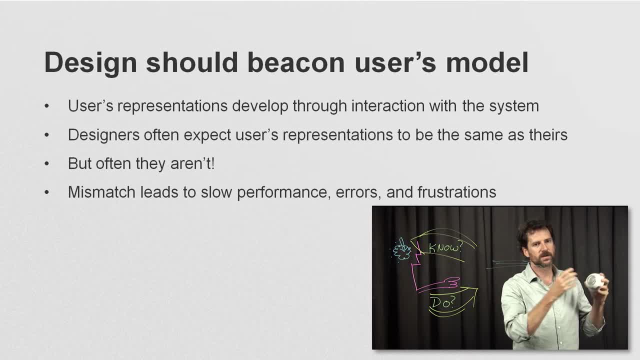 is to be able to beacon what the model of how I do is, what the model of how I know is and what that is. A challenge as things get more sophisticated is that, as designers, we often are, or at least over the design process. 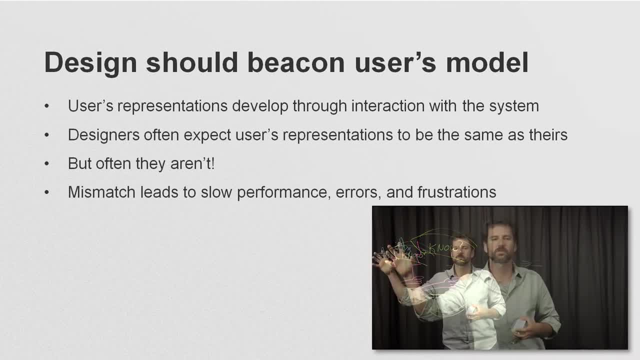 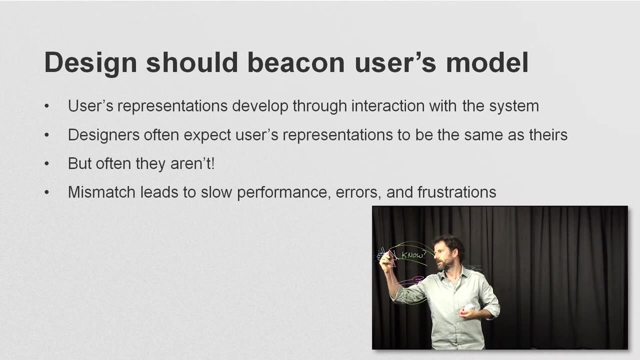 become experts with this technology. We've built these richer mental representations and we expect that the user's representations are going to be like ours, But, as you know, they often aren't, And this mismatch when what's in my head is wrong. 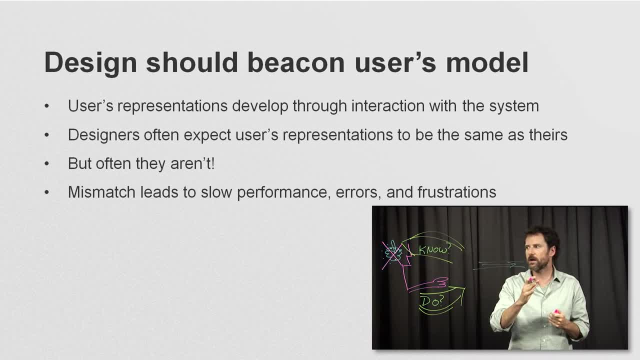 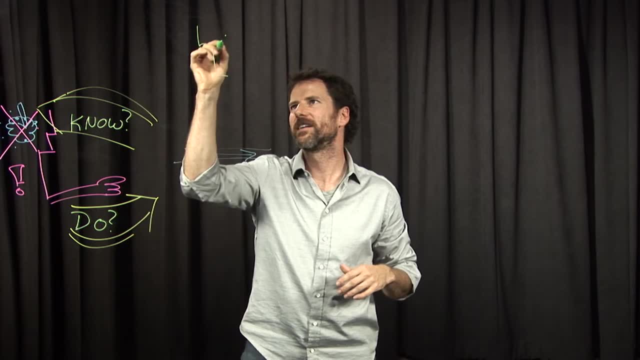 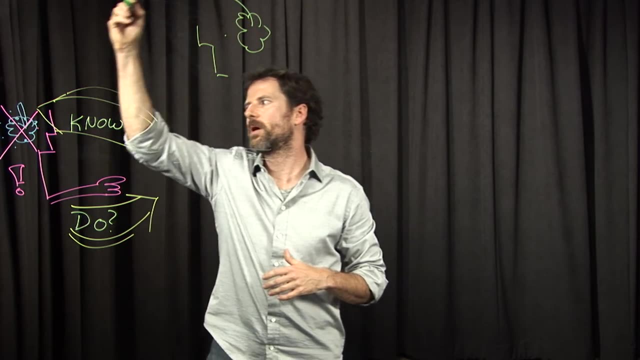 that mismatch can lead to slow performance, to errors and to frustration. The goal, then, as the designer, if I'm over here, is: I want to be able to have a representation in my head. It's almost like you're trying to take a part of your brain. 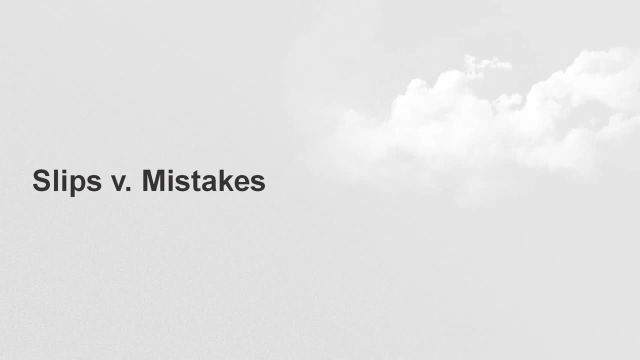 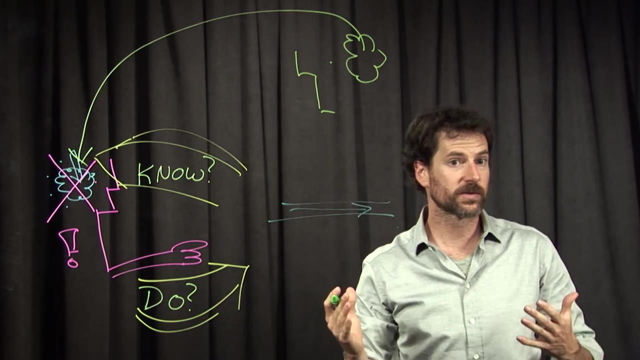 and bring that into the user's head. So if our user makes a mistake, why did they do it? That's essentially the cognitive question about user interface design. Well, using what we just learned, we can ask: did they have the right mental model? 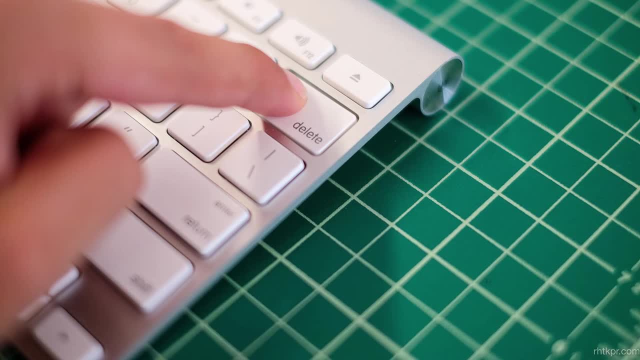 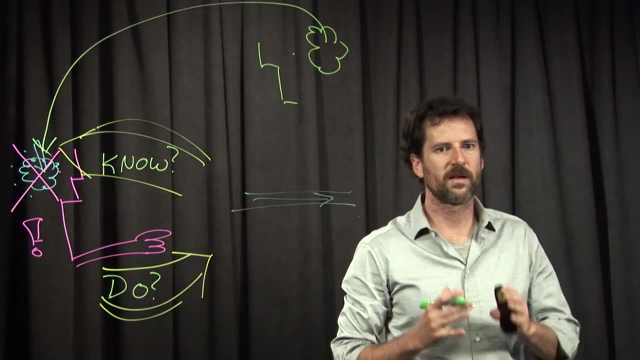 If I'm operating a keyboard type in real fast. I mean to hit the equals key, but I hit the delete key instead. I had the right model. I just slipped. If you're a designer and you're able to understand that something is a slip. 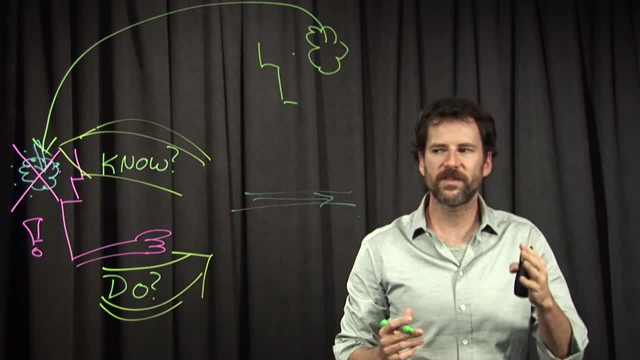 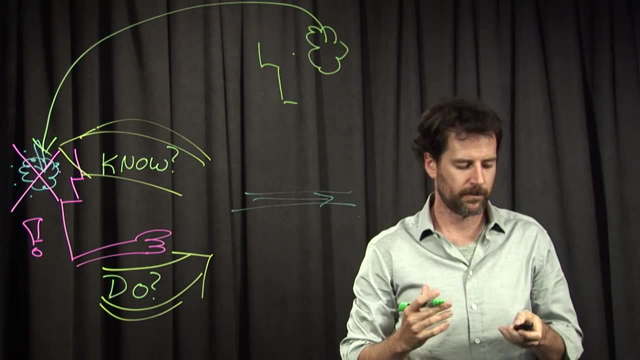 right model, accidentally wrong action. you can fix that with our keyboard, for example. We could spread things out, so it's less likely that you'll hit the wrong thing. You can make the targets bigger- Auto-correct in typing. By contrast, sometimes I can do. 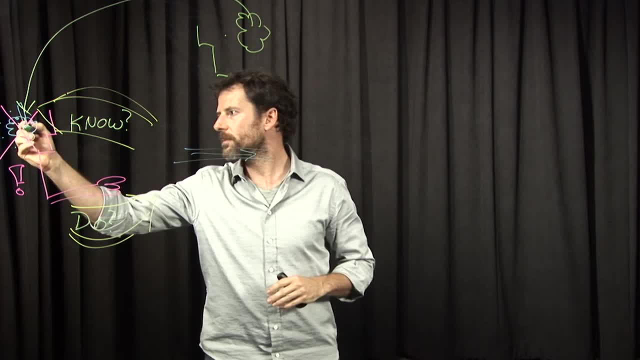 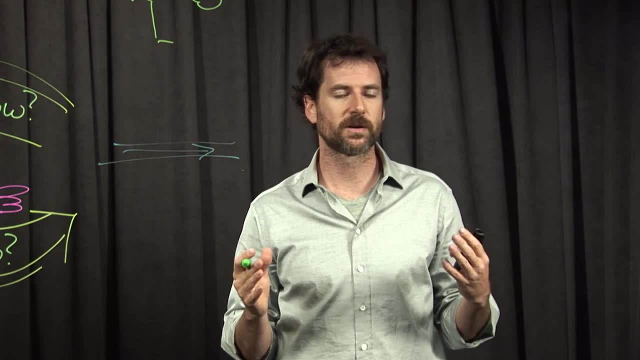 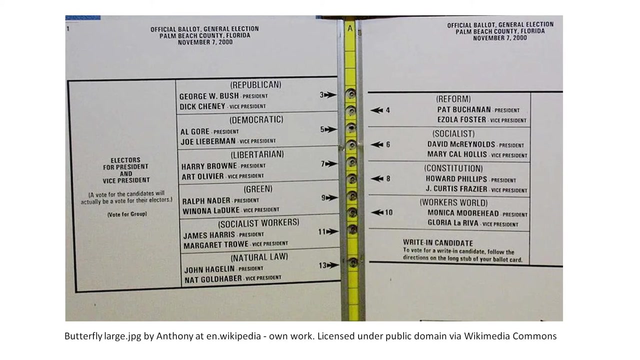 exactly what I intended to do, but I have the wrong mental model. One example of this appears to have happened to a number of people in Florida during the 2000 election. This is what was known as the butterfly ballot. We had a ballot which had names on one side. 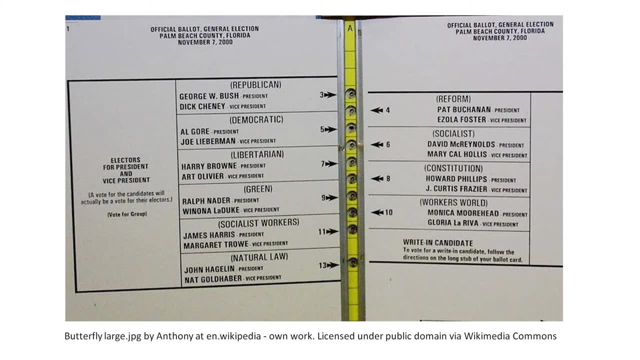 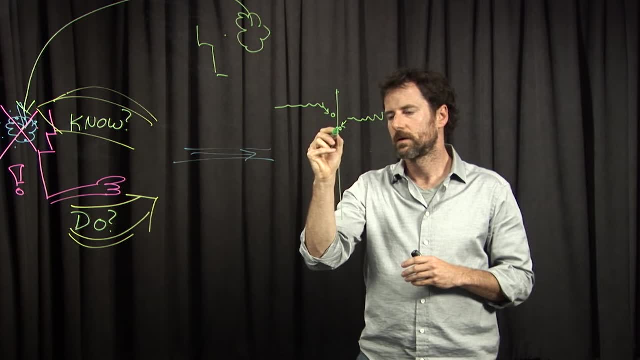 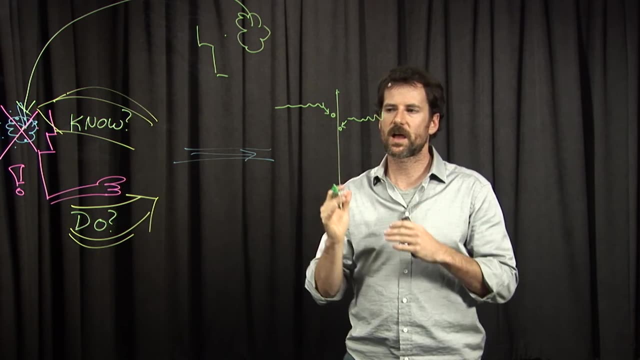 and holes, And the holes didn't quite line up with the names, So there might be a name over here and some people might select the wrong hole. In this case this was a mistake as opposed to a slip, because we knew I hit exactly what I wanted to. 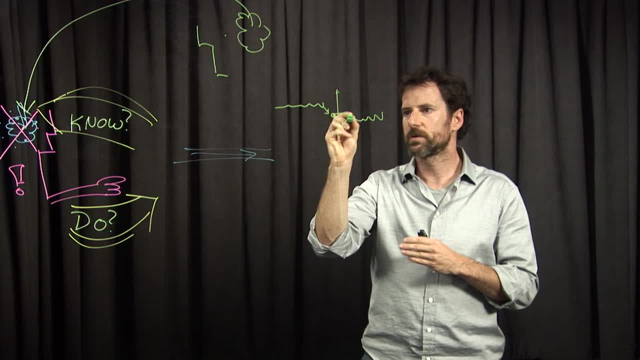 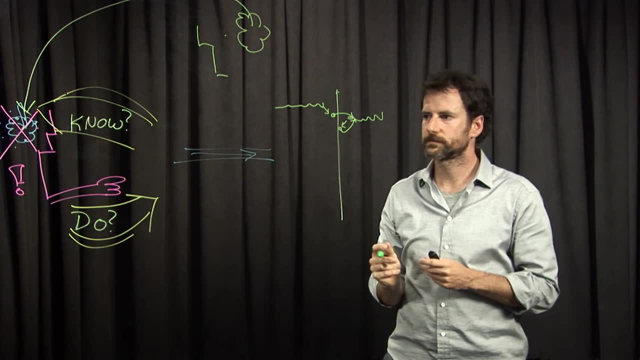 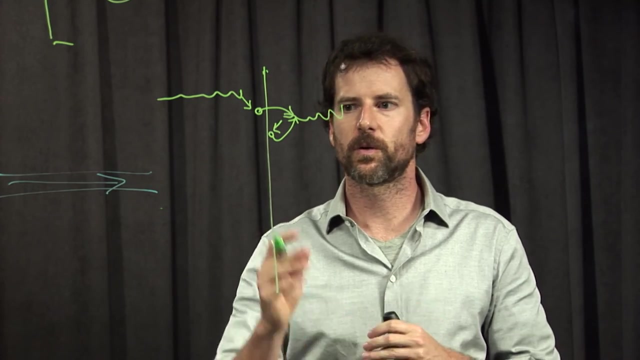 but it was out of the mistaken belief that it corresponded to this when in reality, the tally was being recorded from what should have been this hole. The ballot is also a nice example of how you can use data to be able to infer when people might be making slips or mistakes. 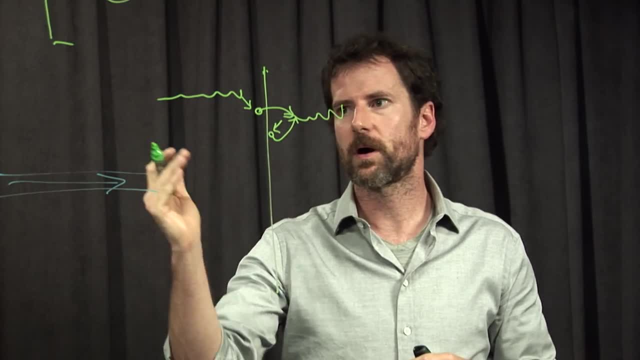 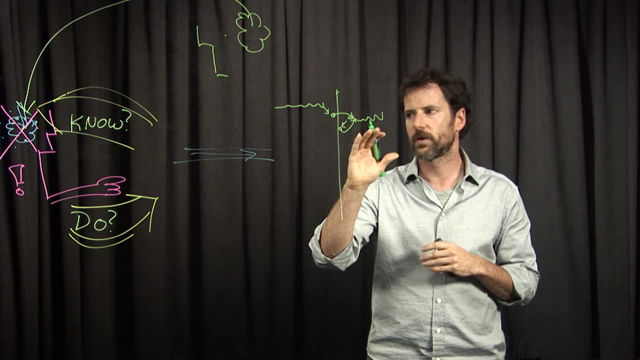 In this case, you had a majority party candidate, Al Gore, and a candidate that, in the rest of the state, received a relatively small fraction of the vote- Pat Buchanan. When Buchanan got an unusually large share of the vote in Palm Beach County. 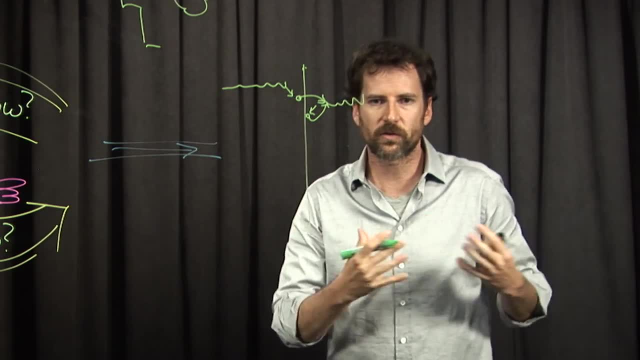 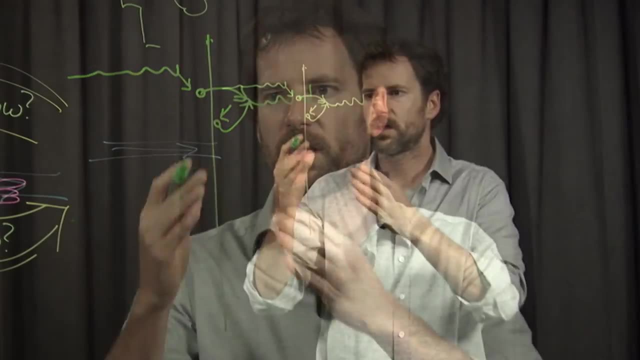 people started to ask why that might have been. So it's a great example of how you can look into the data to be able to make a guess as to where you might look for design flaws Here. when people looked at the user interface that voters were using, 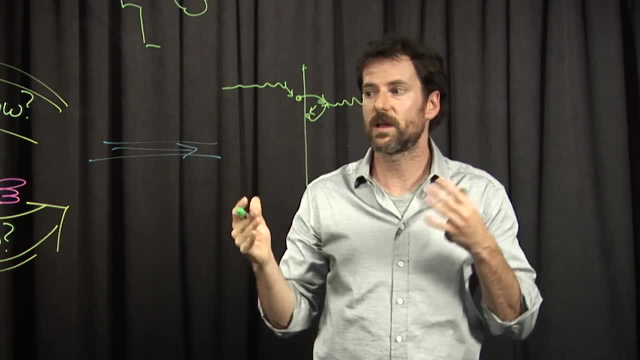 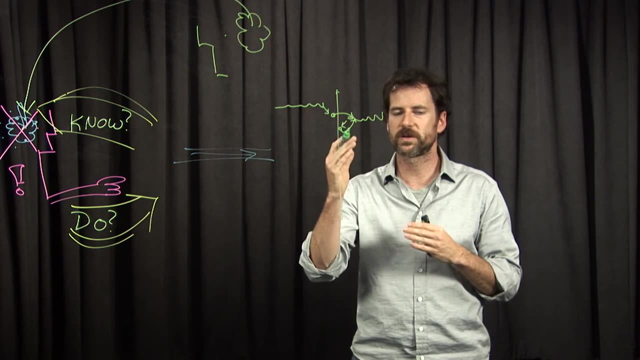 you can see that many people could easily have made an error In this case. 0.85% voted for Buchanan, whereas for a comparison set that number was 0.23%. So you had more than triple the number of people voting for this candidate.